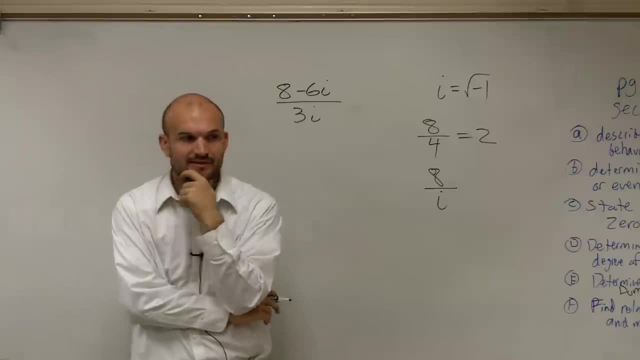 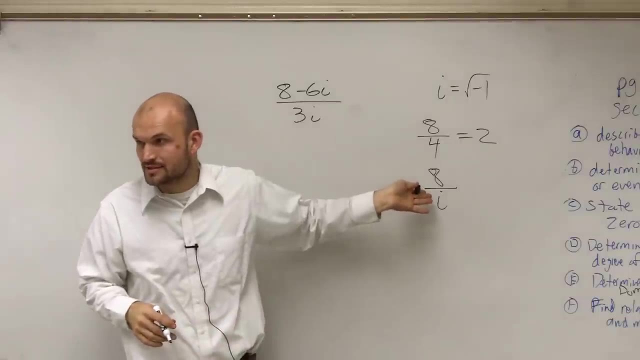 question, right? Well, what we want to do in mathematics is: we don't really want to leave an answer. We don't really want to leave an answer, or even to apply something like this. all right, Because really you're trying to think of an imaginary number. How many times does it? 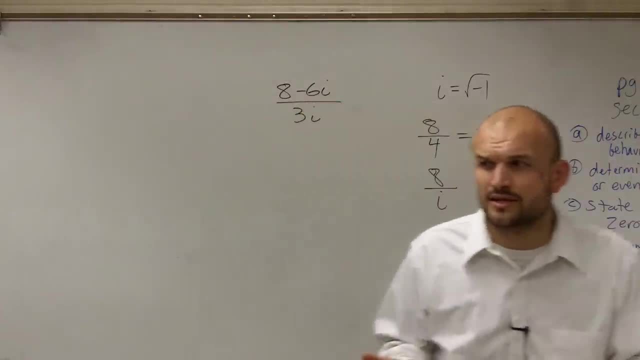 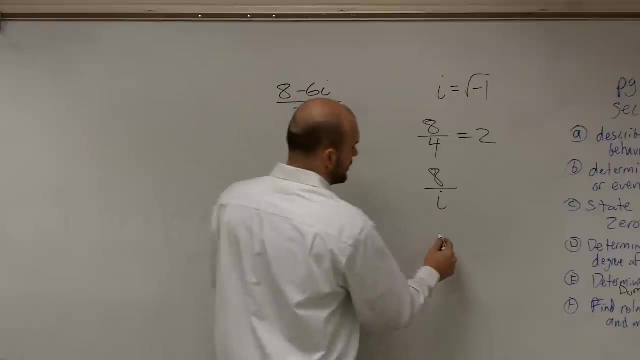 divide into a whole number, Mallory, And that just kind of brings up whole different like other questions of you. know how can we even like explain that or really what's going on? So one thing that we know, the only thing that we know about our i, that's helped. 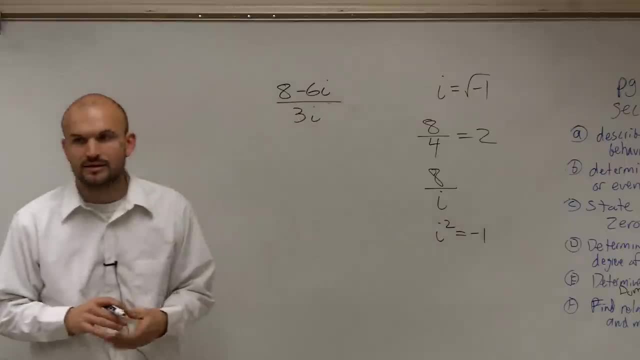 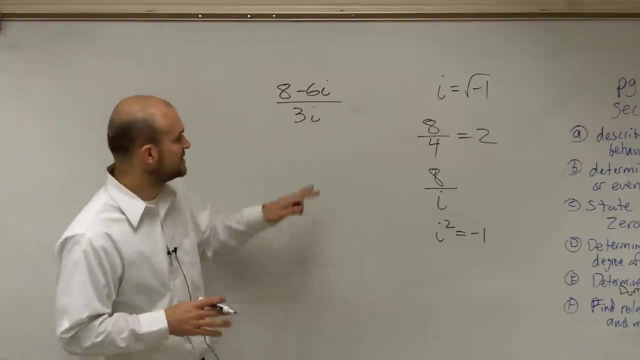 us out is we said i squared is we know that that can represent negative 1, right, Correct, All right. So what we want to do is when we're? we already talked about adding, subtracting and multiplying complex numbers, But what about when we want to divide complex numbers? 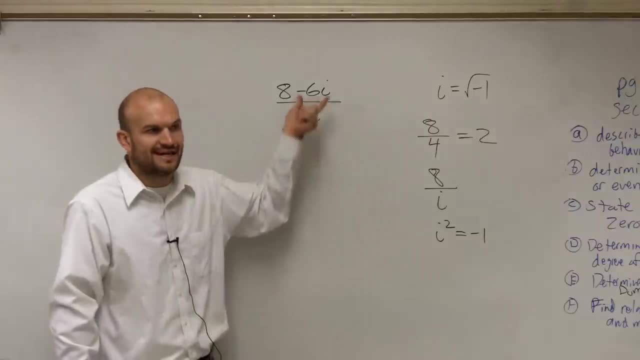 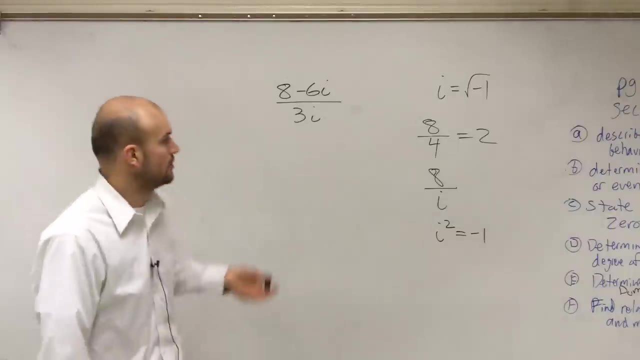 What exactly are we going to do? Because how do you divide something that's imaginary into something else? Well, the thing is, what we're not going to do is we're not going to actually divide it. We're actually just going to simplify the expression. So, rather than actually saying 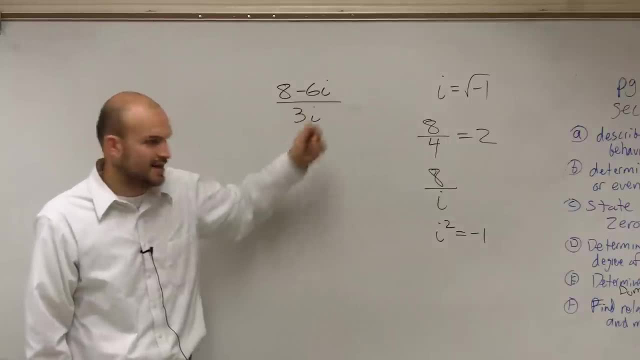 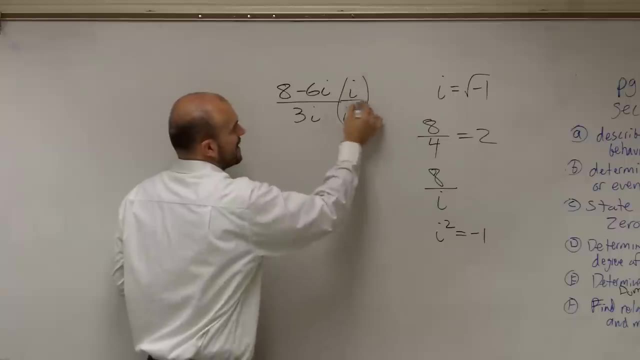 figuring out some kind of number that this divides into. what we're going to do is we're going to simplify it. So, to simplify it, what you're going to do is, if I multiply the top and the bottom by i over i Now, is that okay to do? Can you just multiply any fraction by some number? 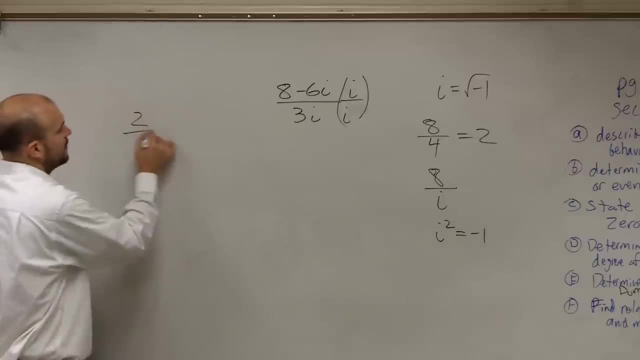 on top and bottom? I don't know. Let's take 2 fourths. You know 2 fourths is the same thing as 1 half right? What if I multiplied by 3 over 3? It still gives the same thing, So do you think it's okay then if? 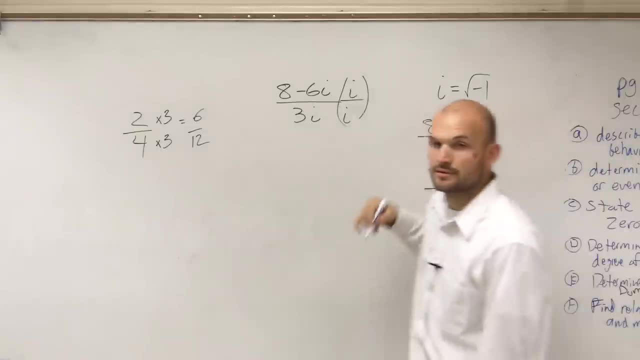 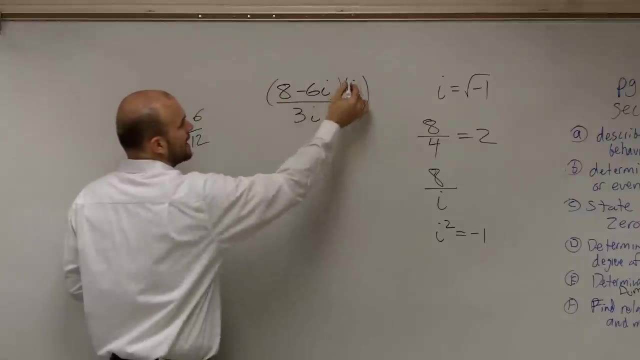 I multiply this by i over i. Yeah, But we have it represented by i, which is okay, right? So if I multiply this by i over i, I now apply distributive property and I get 8 minus 6. i squared all over i. 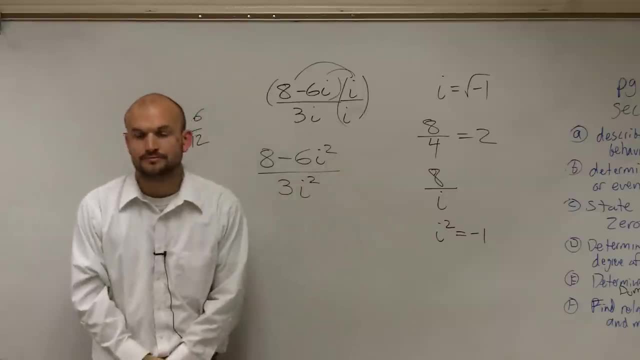 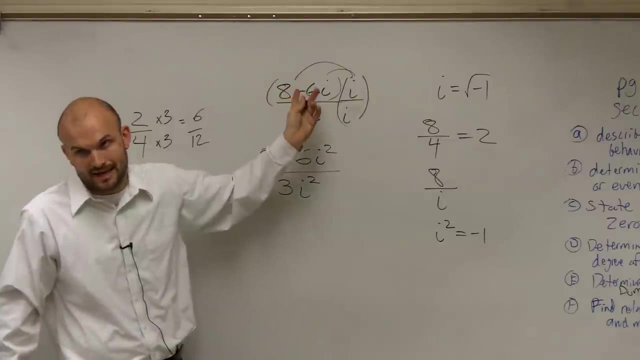 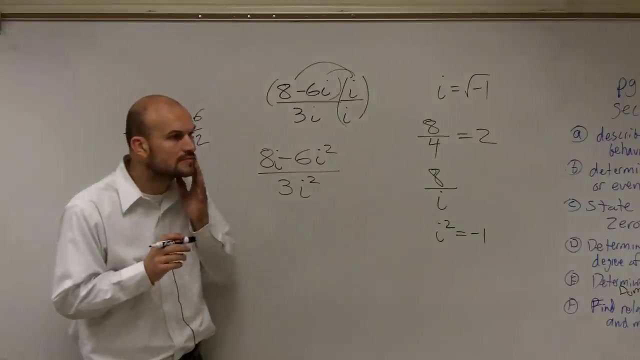 Because, remember, think of this as like a variable. You know, x times 8 would be 8x. So i times 8 is 8,. sorry, 8i, Sorry. Hold on just one at a time. Yeah, So you've got to multiply. i times both of. 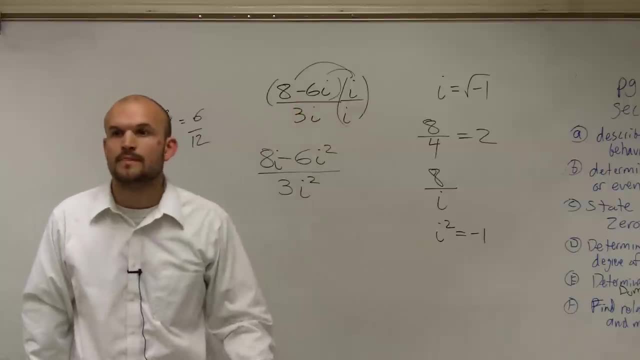 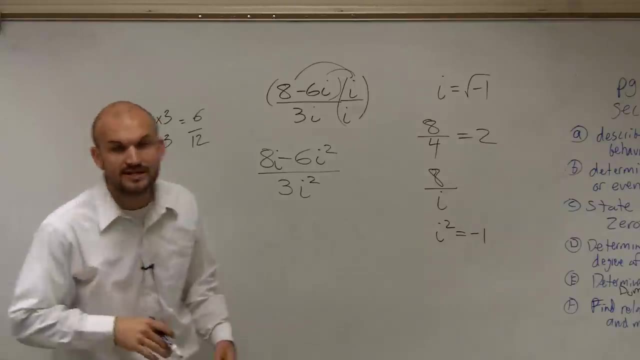 these terms up top and then you multiply i on the bottom. It's so easy, Huh, Why did I do this? Okay, So the reason why I multiplied by i over i and not 2 over 2 or 3 over 3 is: 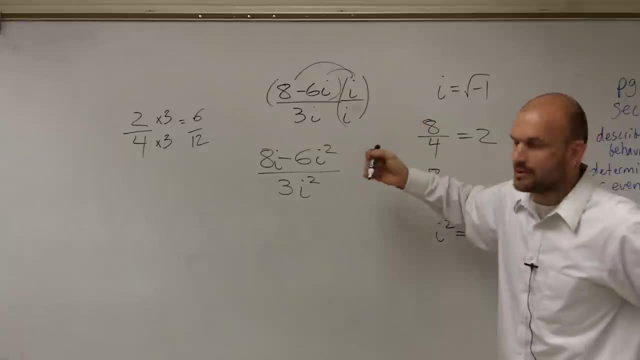 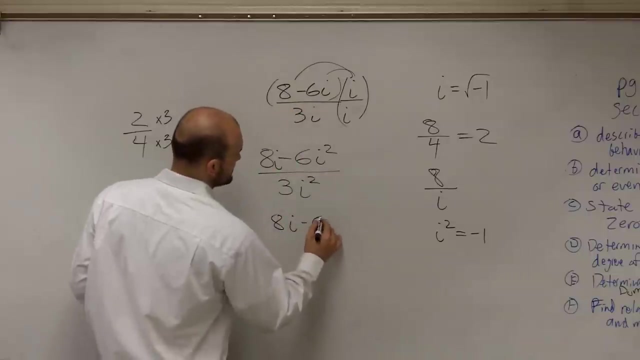 because what happens is you multiply by i over. i look at what you now obtain. You now obtain i squared, And do we know what i squared represents? The negative 1.. So now I have 8i minus 6 times negative 1, divided by 3 times negative 1.. 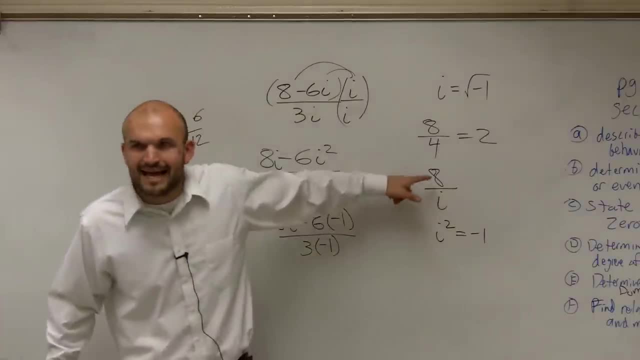 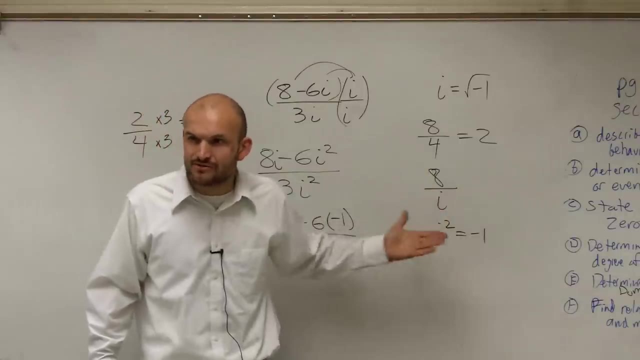 So just by doing this we came up to this question. i divided into 8. That didn't really make sense with us, right? Because you had an imaginary number as your divisor. It doesn't really make sense to divide an imaginary number into something. 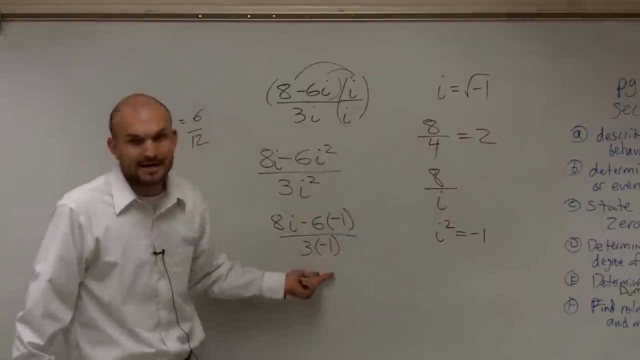 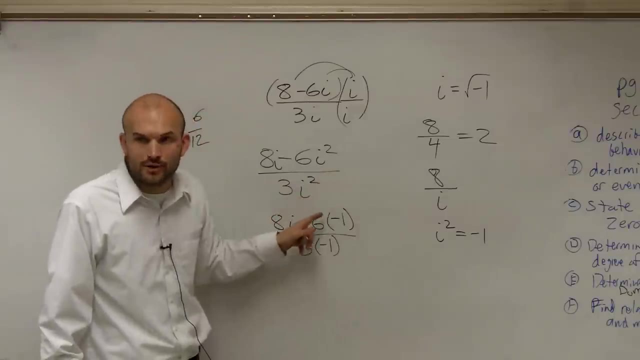 But by multiplying it by i over i do. I now have an imaginary number on my denominator. No, No, I have just negative 1, because we multiply i over, i created i squared, which now gives us negative 1.. Now I can simplify this. 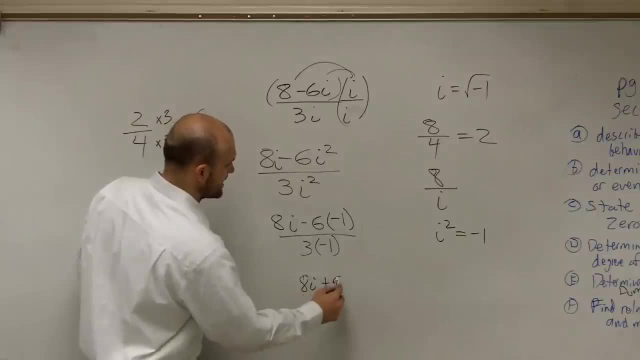 So I have 8i plus 6i squared Plus 6 divided by negative 3.. Look at that, Okay, And the last thing we just need to know is we haven't really gone through it. We'll talk about it a little bit later. 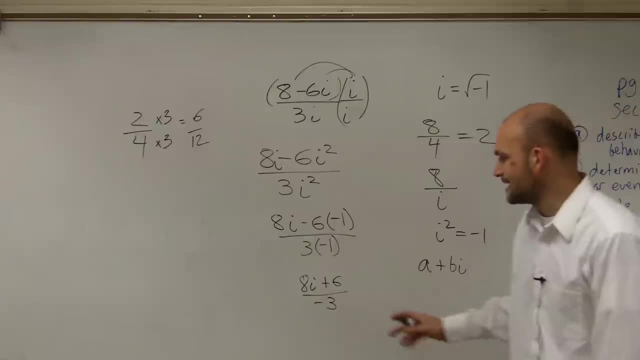 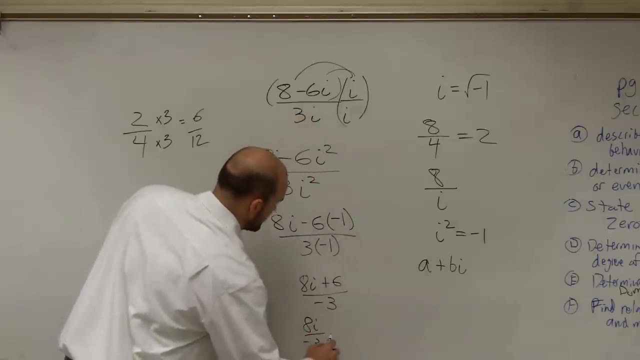 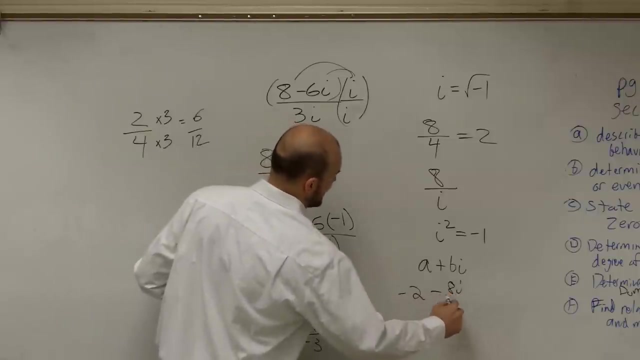 But complex form of numbers is a plus bi. So the final answer for this would be: you're going to separate this into 8i divided by negative, 3 plus 6 divided by negative 3.. So your final answer is going to be negative 2 minus 8i over 3.. 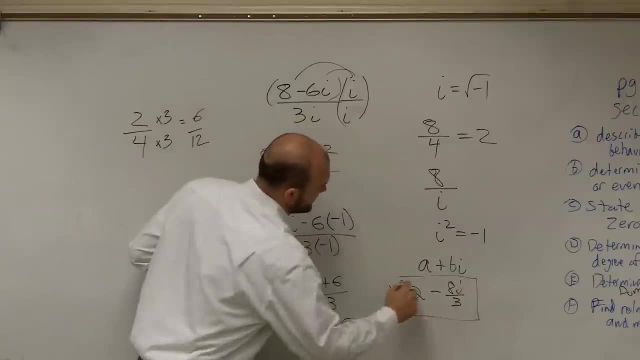 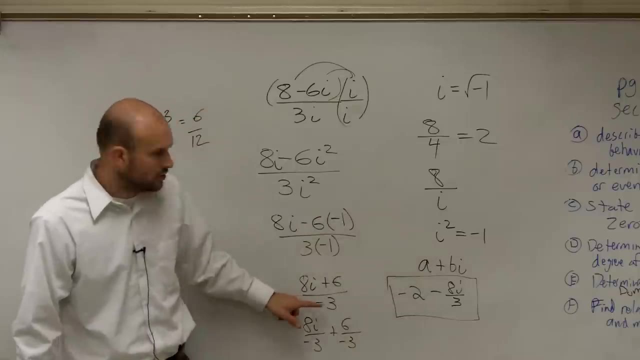 Wait what? Why would you do that? We haven't really gone into writing complex numbers in complex form, But this is your standard complex form. We don't want to finish your answer like this. We like to write it in a plus bi format. 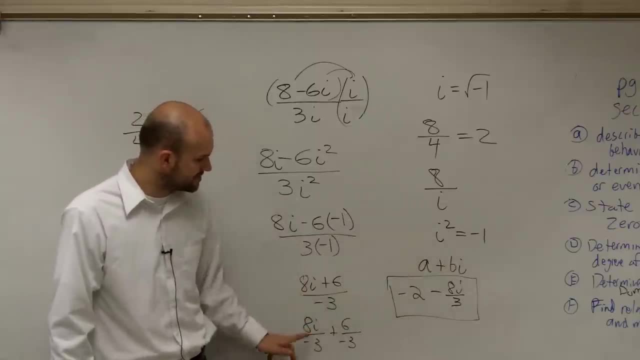 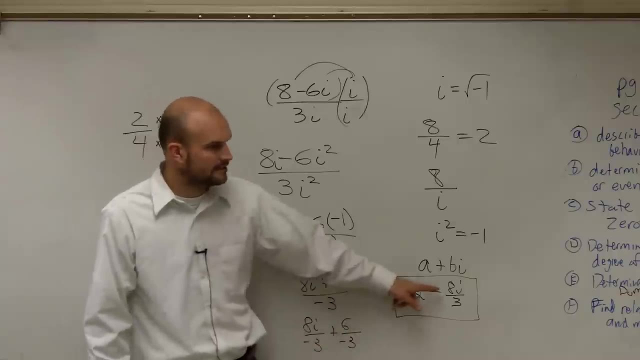 So what you do is you take your divisor, divide it into both terms, And when I do that, I can simplify this: 6 divided by negative 3 is negative 2.. And I can't simplify 8i over negative 3, so I just write it like that, Yep. 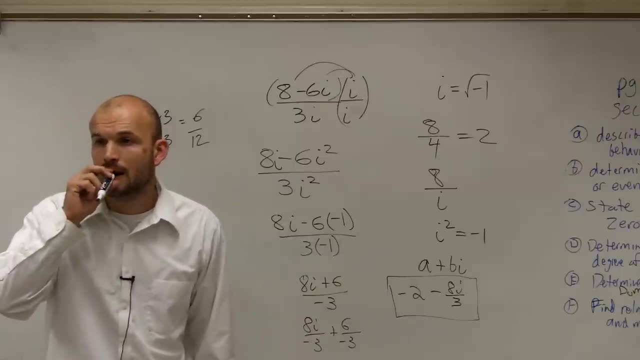 Any last questions. You mean using square root of negative 1 instead of i. Yeah, There you go.